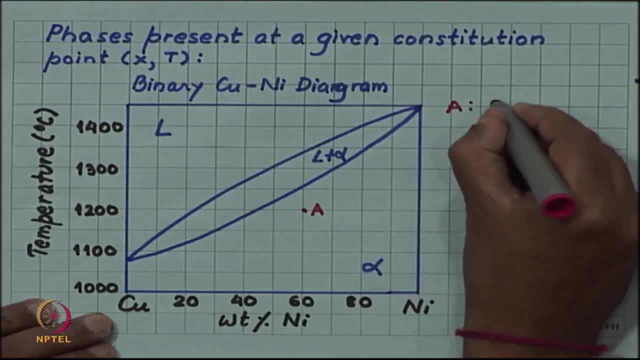 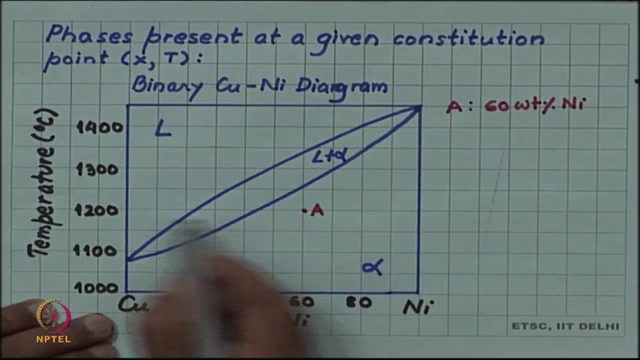 I look at its x component, that is 68 percent nickel. So if I look at its x component, that is 68 percent nickel. So if I look at its x component, that is 68 percent nickel. So this means it is an alloy of 68 percent nickel. And if I look at the y coordinate, its 1200. 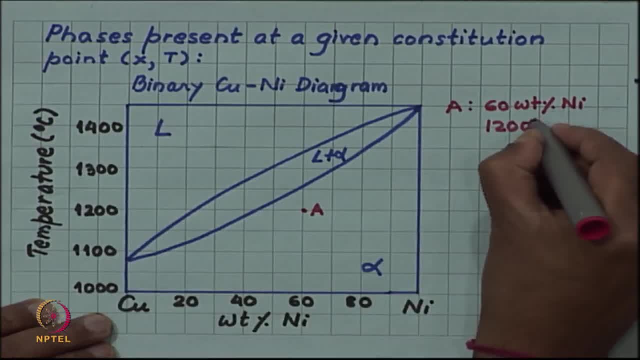 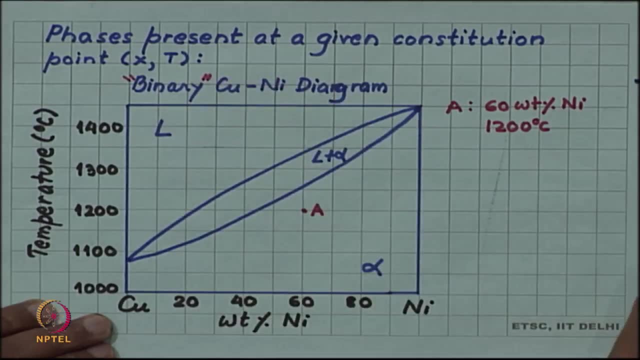 degrees Celsius, So a 68 percent nickel alloy. and I am only writing 68 percent nickel because we have binary alloy. So this is the convention in binary alloy, since the other component obviously will be 100 minus the component which you have given. So for example, 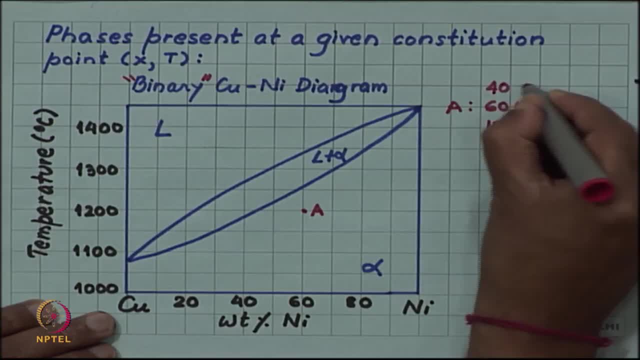 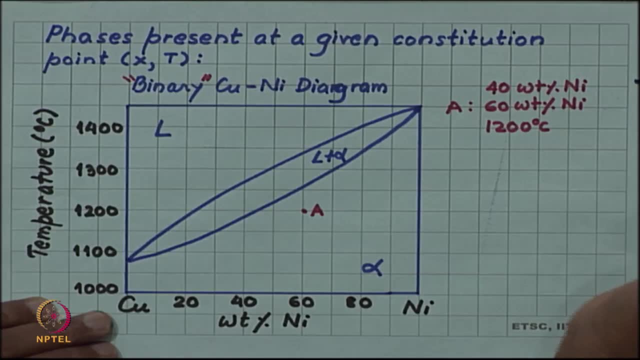 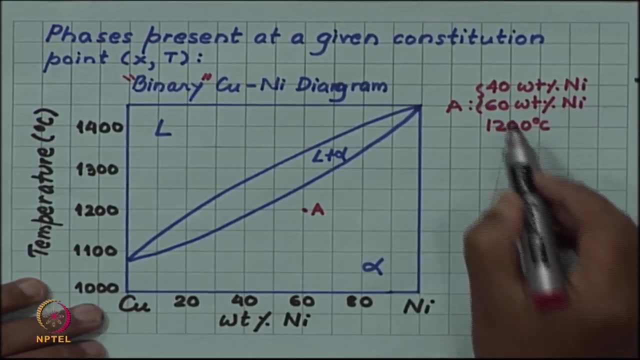 68 percent nickel. nickel automatically means that it is 48 percent copper. So if you show this you can write. but giving one component, the proportion of one component, is sufficient to define the composition for binary alloy. So we have 68- sorry, 48 percent copper, So 68 percent. 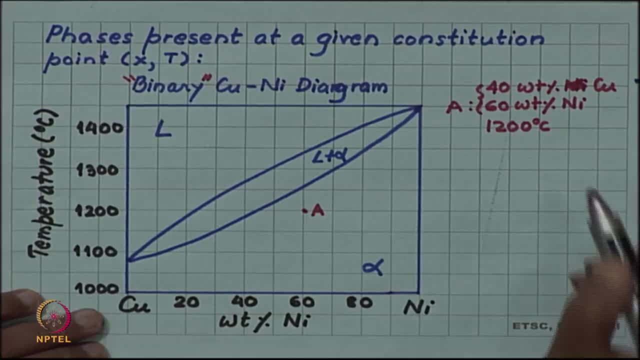 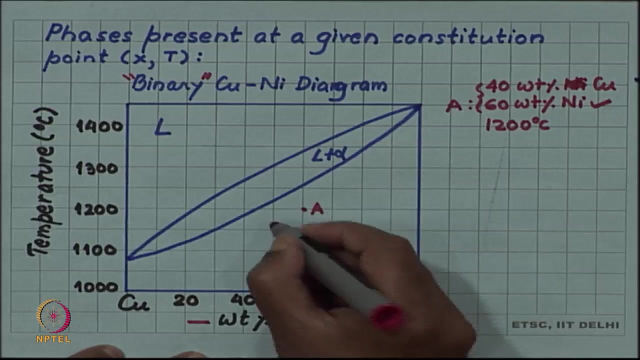 nickel, 48 percent copper. either of them you can give, but we, since we are saying that we are using weight percent nickel as our composition axis, So we will give 68 percent nickel as the composition of this alloy. So this is my point and the alloy has been. 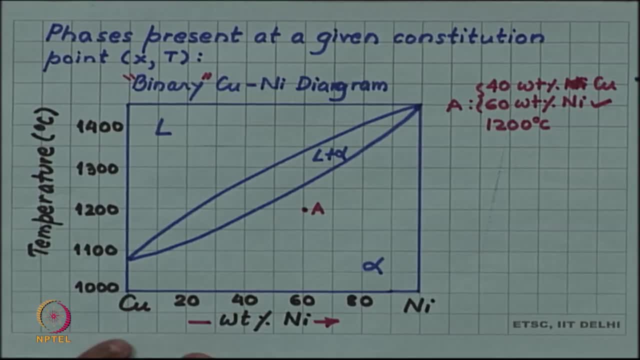 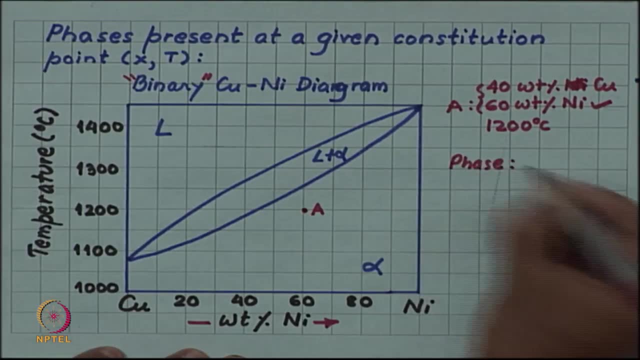 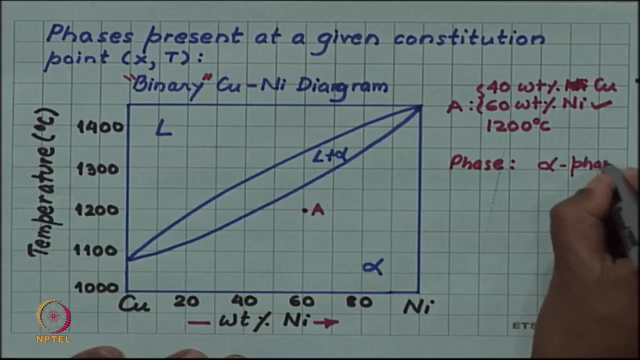 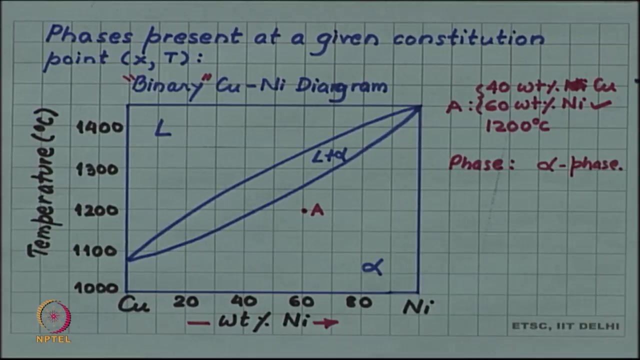 equilibrated at 1200 degree Celsius. So the question: what is the phase here? All you have to do is to see in which region it is falling. since it is falling in the alpha region, we will say: Let us say that this is an alpha phase. phase is alpha phase. Now let us look at another. 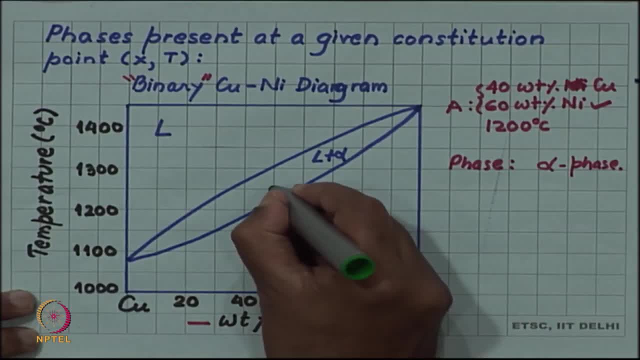 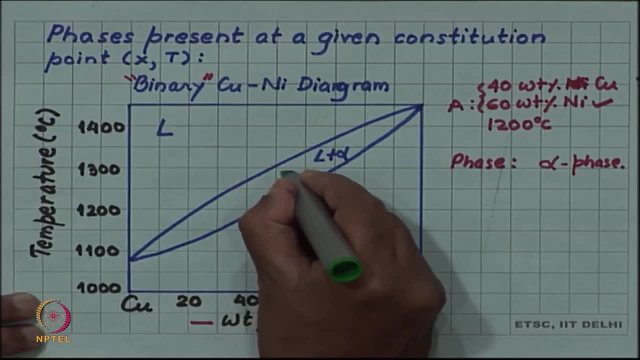 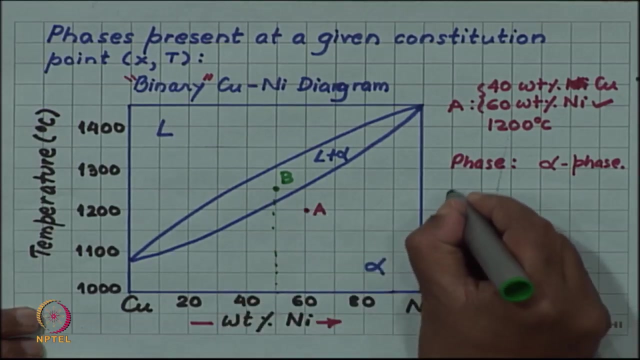 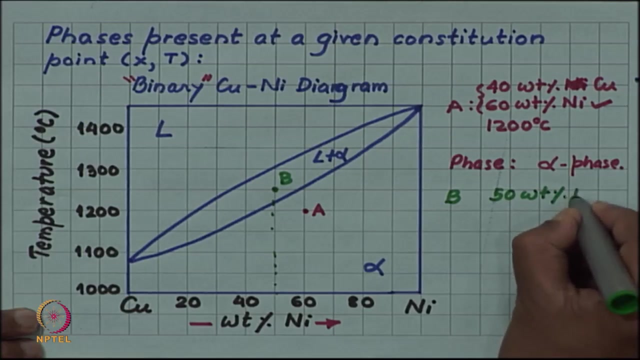 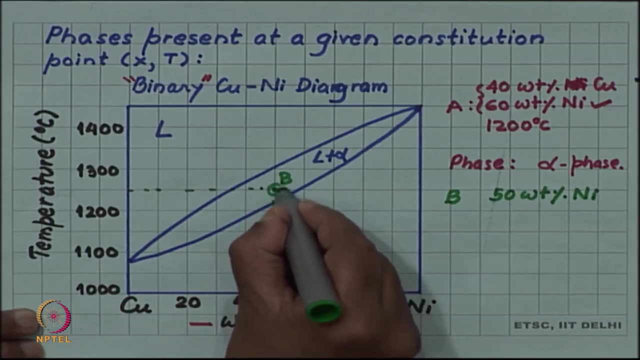 alloy. let us look at this one, alloy B or constitution B. So if we now look at its x component, that is 50.. So the composition is 50 weight percent nickel, So it is a 50-50 alloy. and if I look at the temperature, I find that it is 1250. 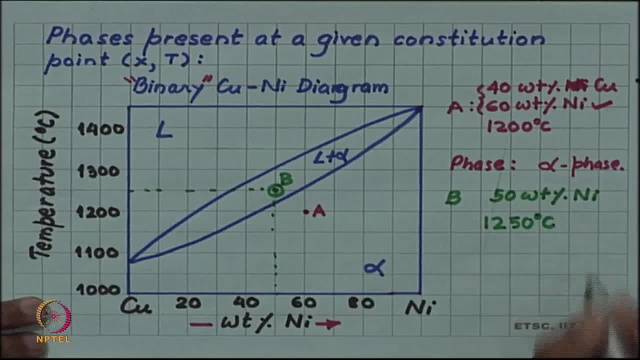 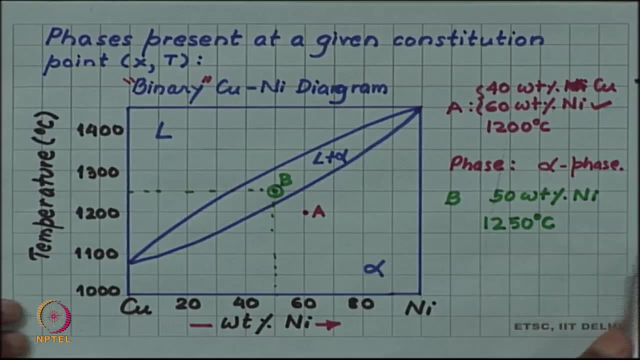 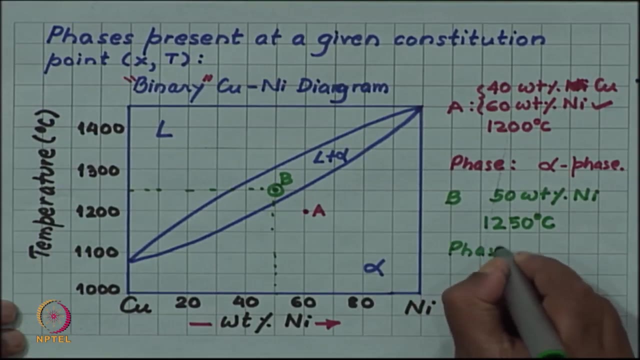 degree Celsius. So an alloy of 50 weight percent nickel, 50 weight percent nickel, 50 weight percent copper is being headed at 1250 degree Celsius. So what are the phases present? So this time we get a little bit more interesting answer, because now it is. 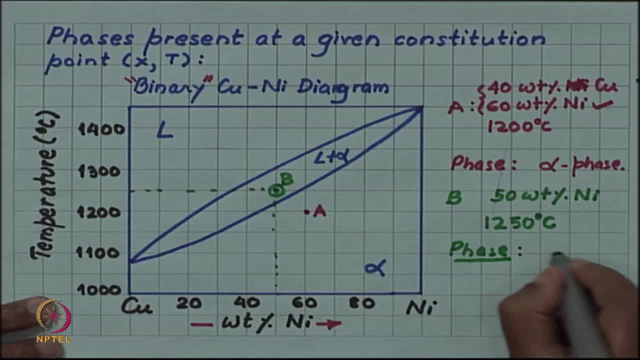 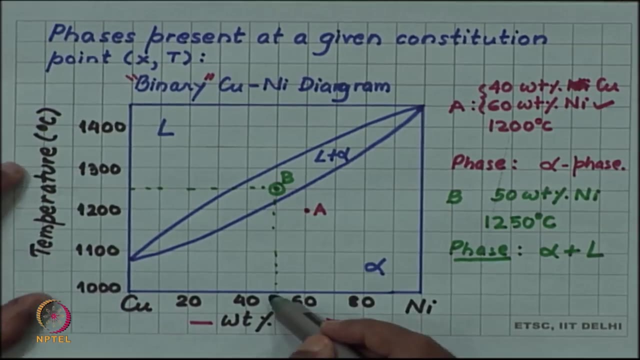 falling in the two phase region. So we will find that two phases are present in this alloy, So both alpha and liquid are present at this point. So at this point, if I take such an alloy and heat it to 1250 degree Celsius and hold, 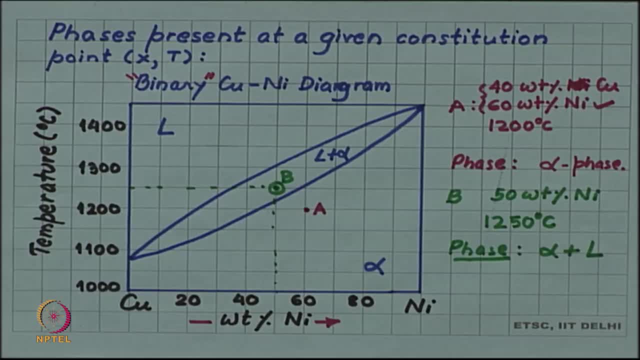 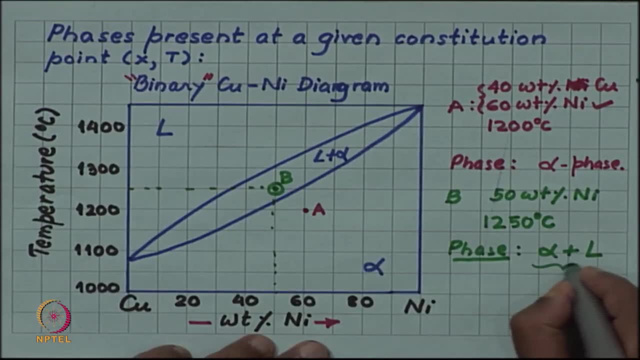 it in equilibrium at. that means I wait for long enough time for equilibrium to be achieved. then I will find that alloy is a mixture of two phase, two phases, So this is a two phase structure. This is the basic function of a phase diagram and this is something which 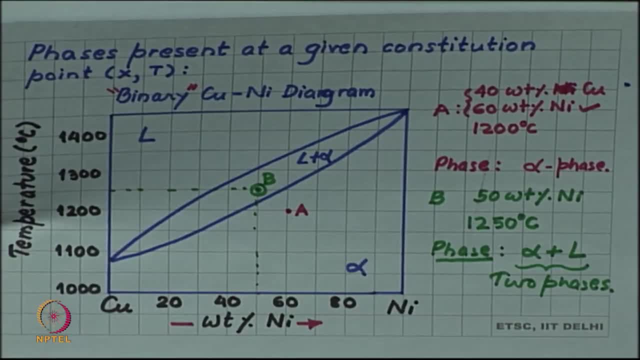 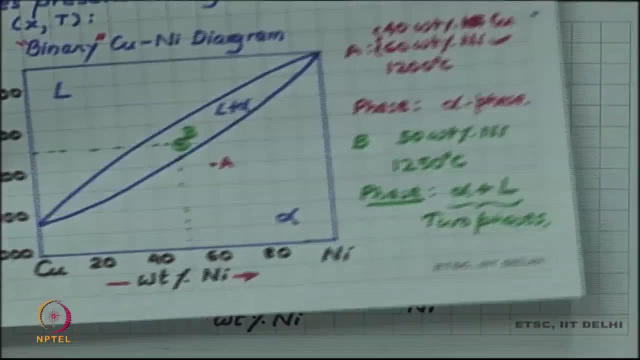 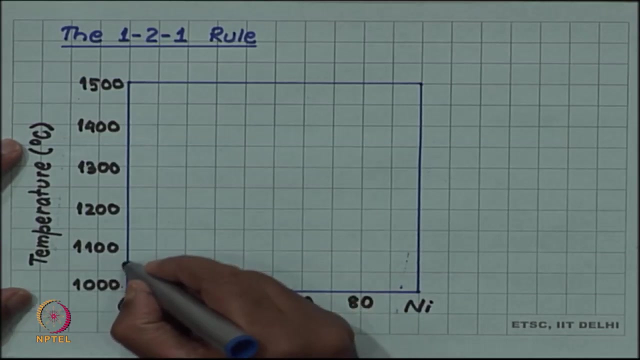 phase diagram can vary And very easily answer. you just have to look at the plot, the point of your interest on the phase diagram, and read the phases present. An interesting thing which happens when you so let me draw the boundaries. So an interesting thing which happens when. you. 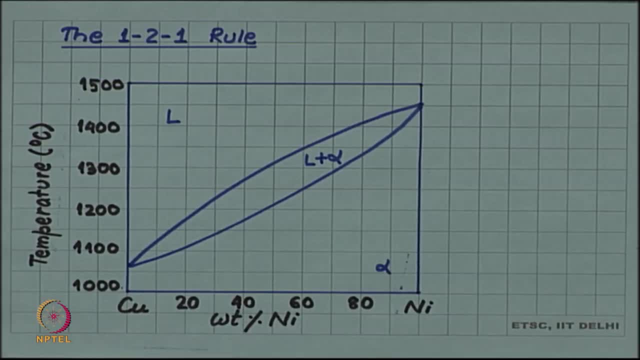 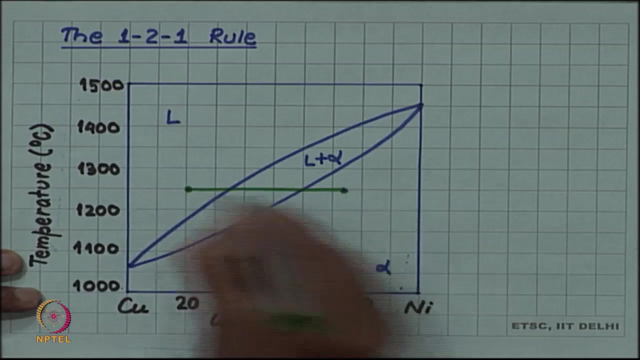 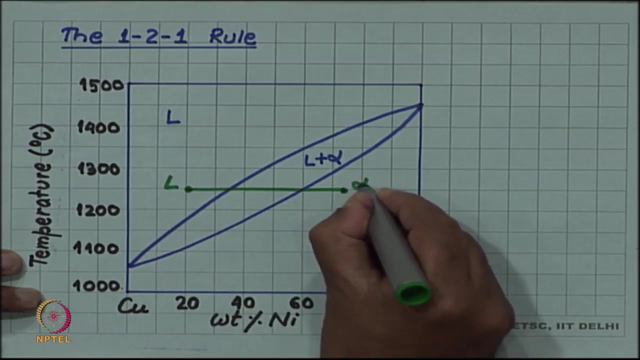 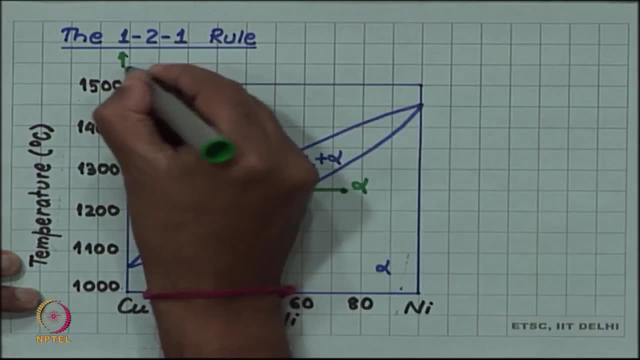 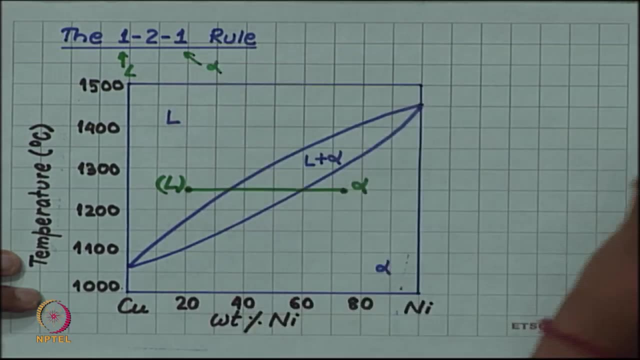 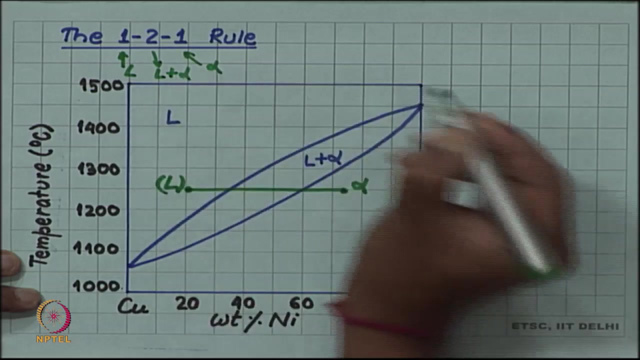 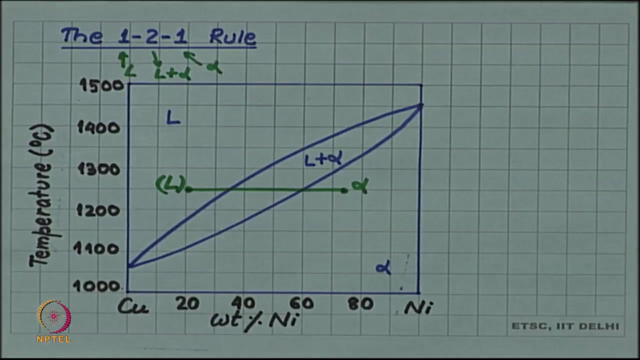 that I have a one single phase, in this case liquid. at another end I have another single phase, alpha. then in between there has to be a region where mixture of these two phases should be present. So liquid plus alpha. so this is always true in a binary phase diagram. 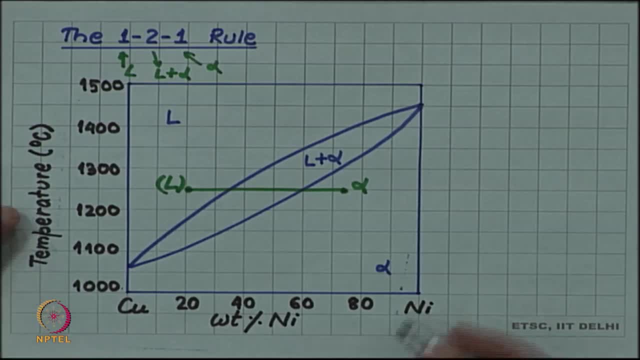 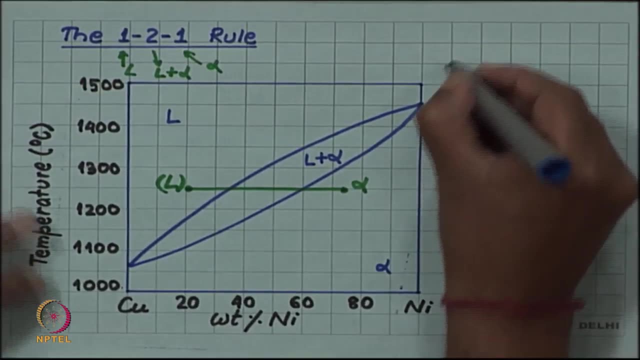 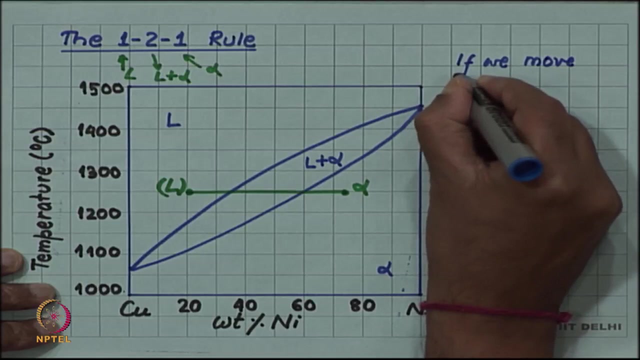 and we call this with a name, one to one rule, although this name is not very common in literature, but we will be using in this course, So let me write this down. if we move horizontally means, since our Y axis is temperature, moving horizontally is moving along an isotherm. 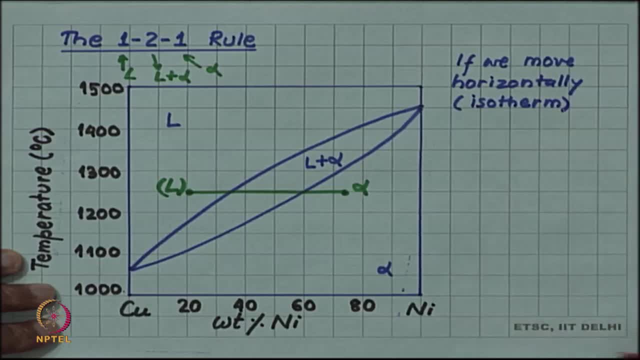 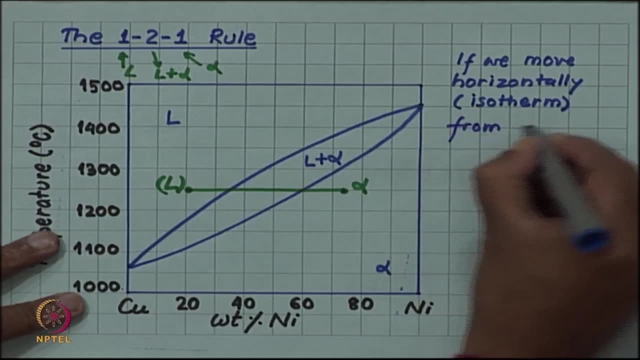 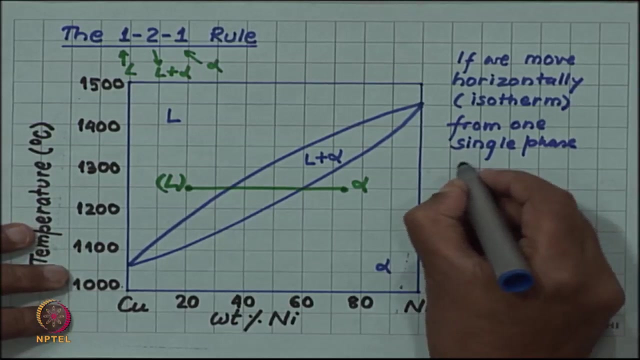 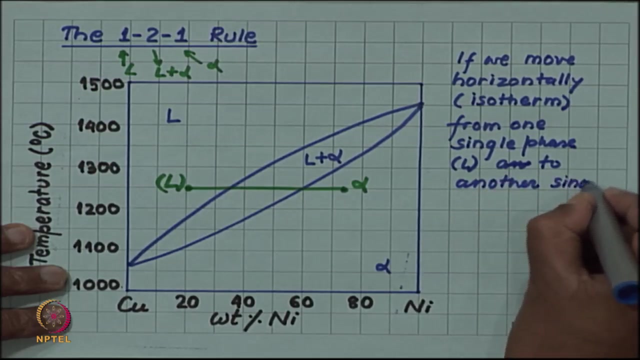 Okay, So if we are moving along an isotherm from one single phase- one single phase in this case, let us say example liquid- to another single phase, in this example, alpha. So this is for example, it can be any phase, example liquid, example alpha. 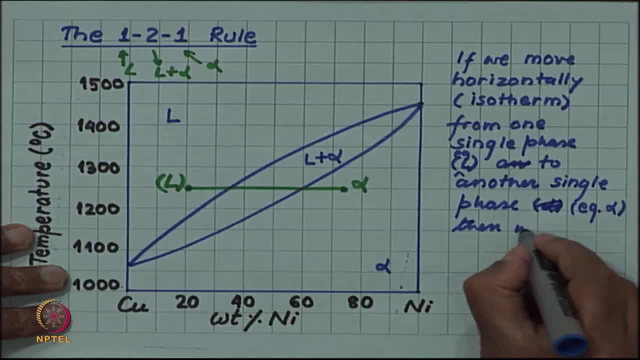 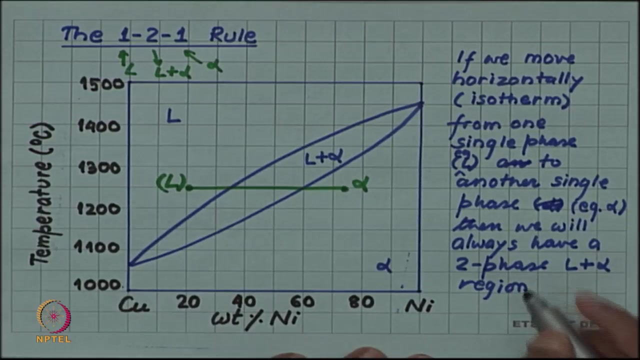 Then we will always have a two-phase liquid plus alpha region, whatever that single phases were there. So if one phase was alpha, another phase was beta, then the two-phase alpha plus beta. So the two-phase alpha will be present. So we will always have a two-phase region in. 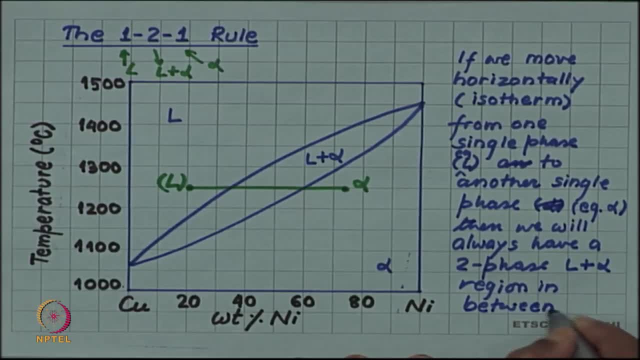 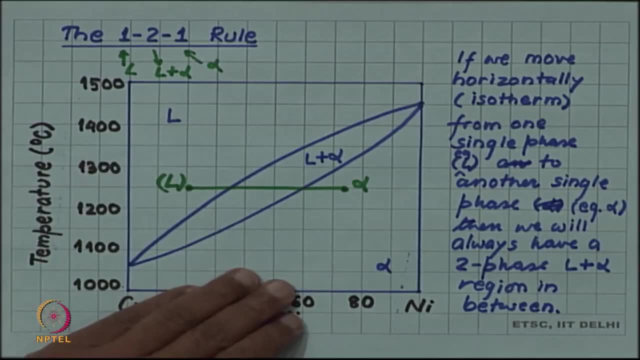 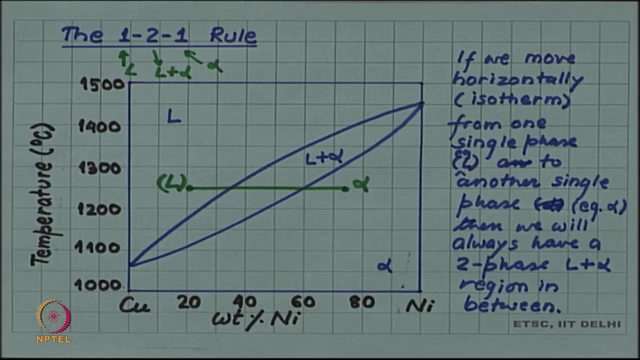 between. So this is important- and in fact many standard phase diagrams which you will come across in the literature Many times they will list only the single phase region, because the two-phase region always can be found as the combination of those two single.